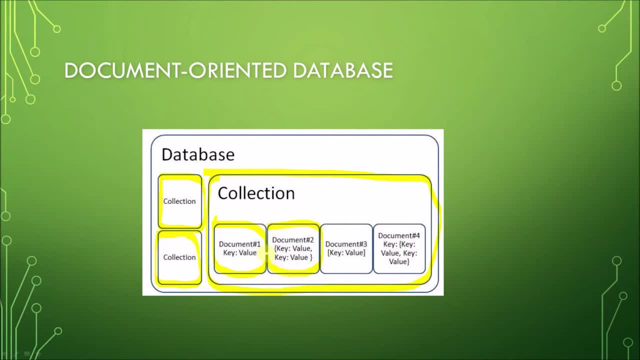 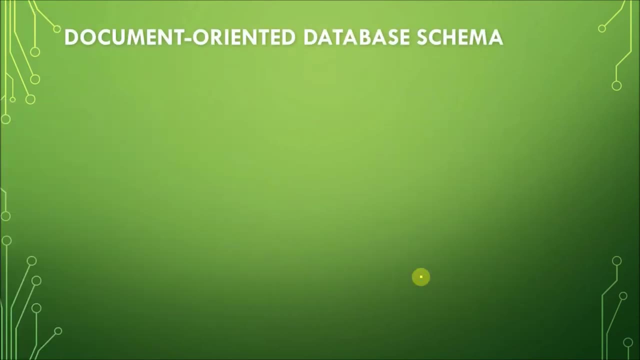 So we have documents. So we have one document, another one and so on. Now these documents follow a certain format. In this example here we have JSON format to describe the document. Now let us compare and convert a relational schema with a document database schema. 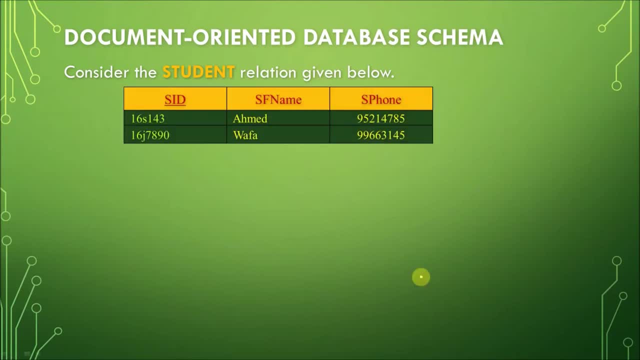 If we recall, in a relational database system you must define a schema before adding records to a database, right? So in this example here we have a student relation with three columns or fields and two records or rows. Now let us convert this student relation into a document-oriented schema following the JSON format. 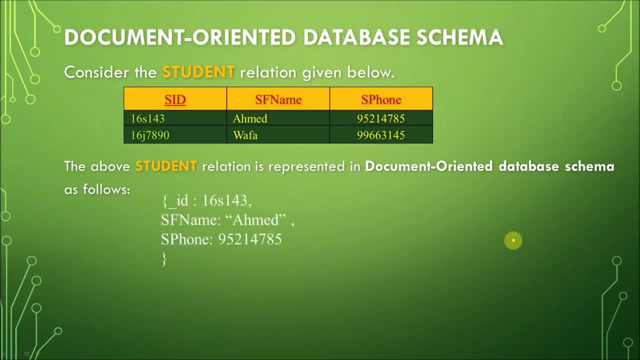 The above student relation is represented as follows: So this would now be the schema for the student relation. The first entry here would be for the student 16S143.. So this is one document in here, and the second record, about 16J7890, is now written in this document. 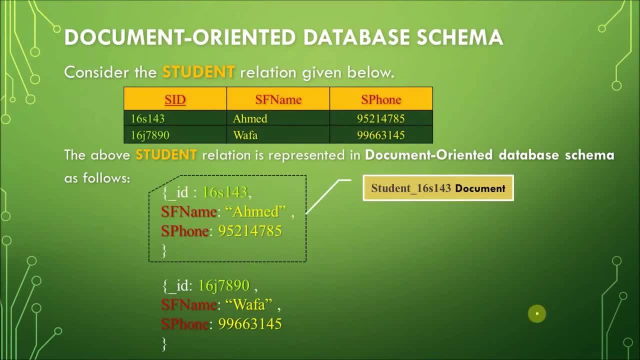 So again, this would be one document for the student record 16S143.. As you can see in here, this is the primary key. Depending on the format chosen, this is how it would look, like An underscore ID colon for the primary key and then the value of the primary key. 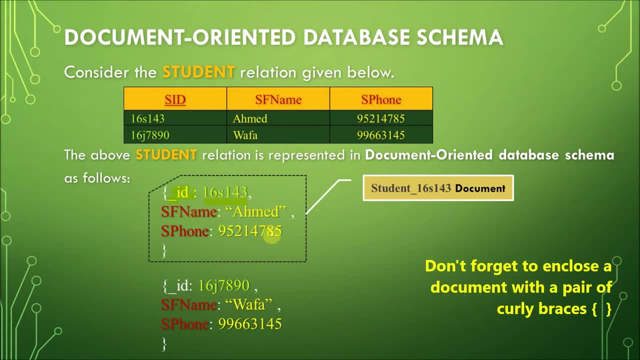 and then a comma to separate one value or one attribute from another attribute. So this is the record of 16S143, Ahmed. You put the column name here and then the colon symbol and then the value for SF name. In this record we have, or in this document we have, Ahmed. 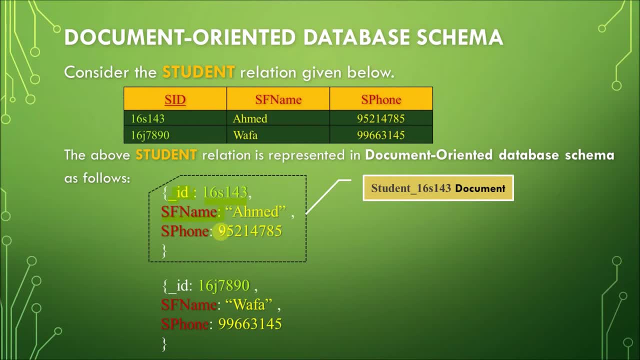 And then another comma to separate again one field from another field. So the next field is Sphone. So we have Sphone here and then a colon symbol and then the value of the Sphone. So this is the ID, the primary key, SF name, and then the phone. 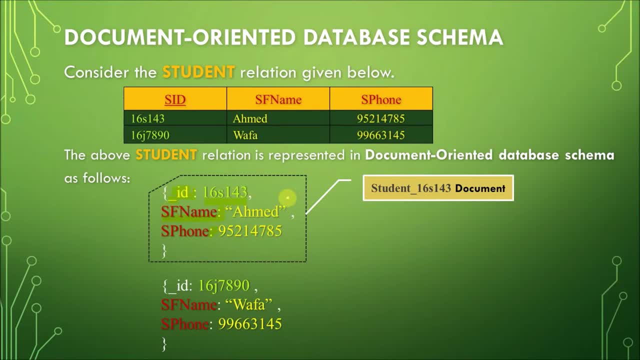 This would form one document. Again, one record in a student relation or table would be one document in a document-oriented database. The second record is about the student 16J7890.. So again we have underscore ID colon and then the value for the ID, the primary key here. 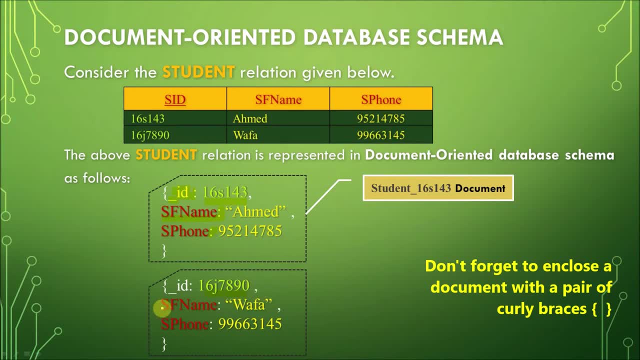 Separate it with a comma, and then the next field or column SF name, the value, which is Wafa, And then a comma, And then the next field or column name, which is Sphone, And then the value is 99663145.. 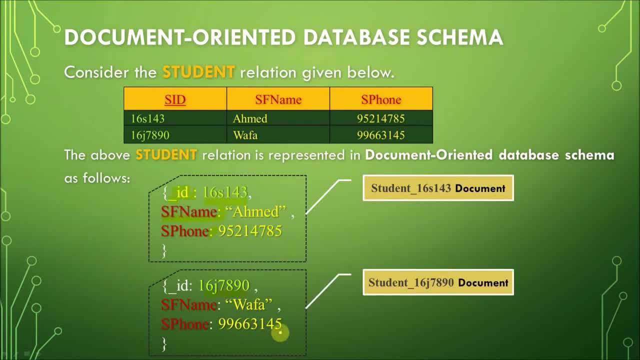 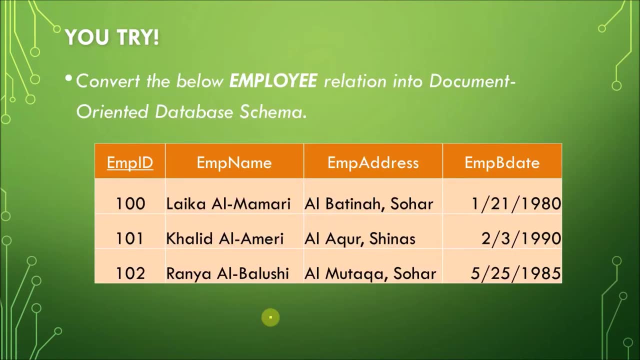 Again, this would form the next document, which is about the student 16J7890.. So there are two documents in this collection. Now let's try Convert the below employee relation into a document-oriented database schema. So this is a relational schema, an employee relation with four columns and three rows. 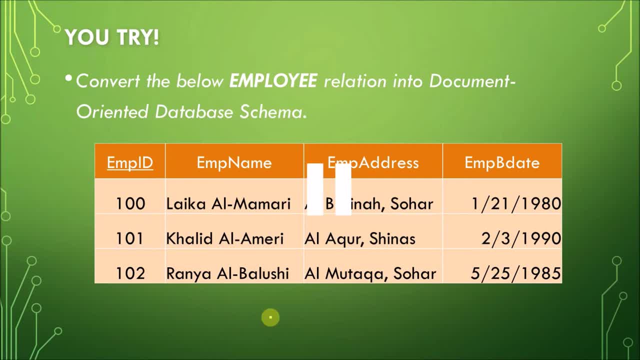 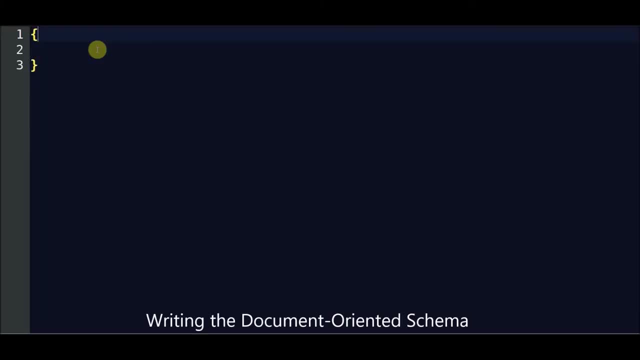 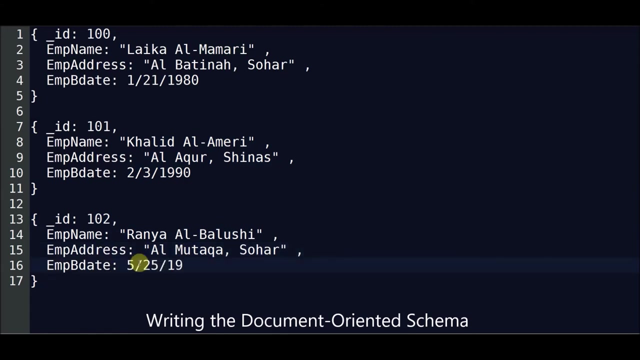 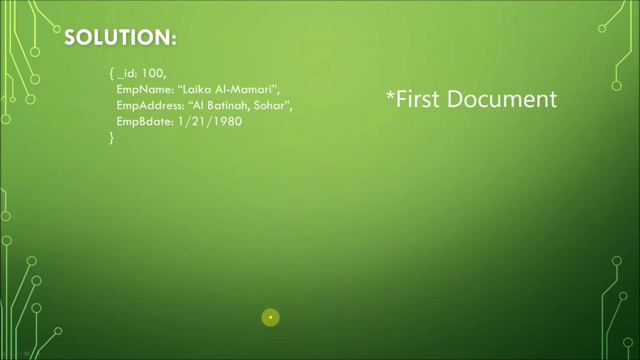 Now take your time and pause this video, Are you done? Let's see the solutions. So this would be the first record about employee 100.. So this would be the first record about employee 100.. Okay, The next one would be another record for employee 101.. 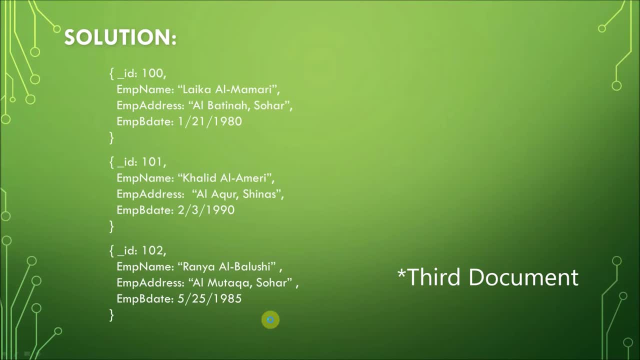 And this one would be for employee 102.. Now let's take a look into the details Again. employee 100.. Note that we have a curly braces in here opening curly braces underscore ID for the primary key. This would be the somehow key colon, and then the value here is 100..